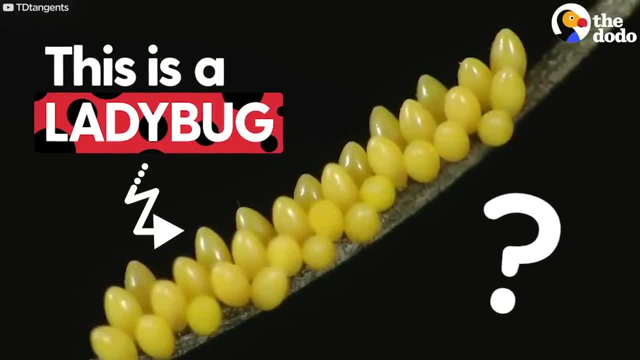 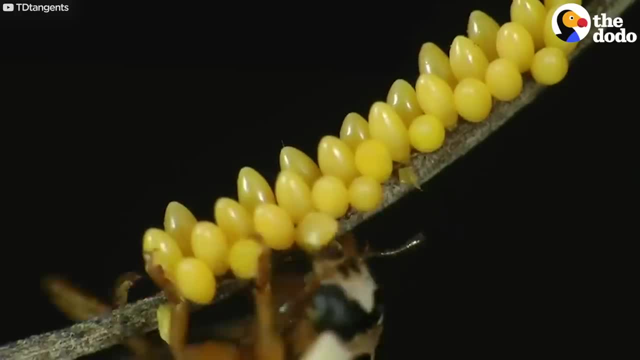 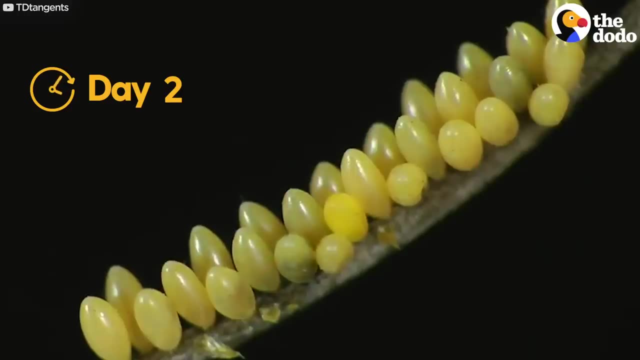 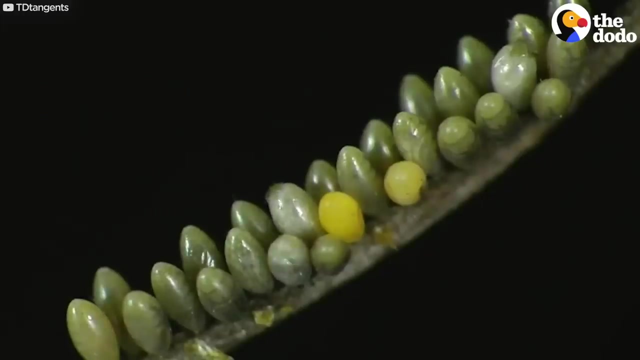 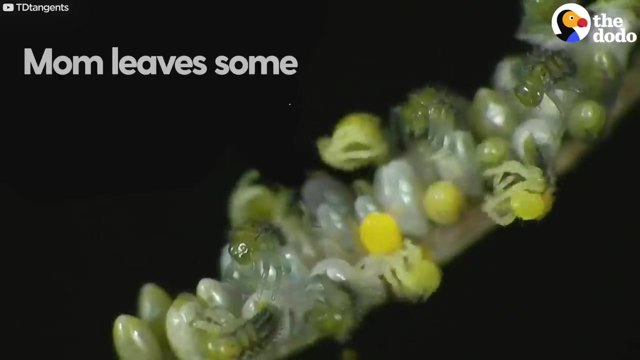 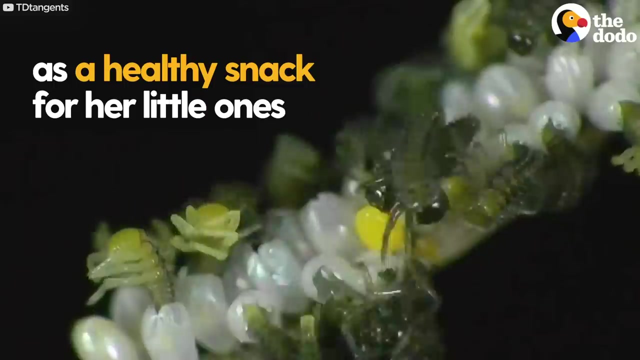 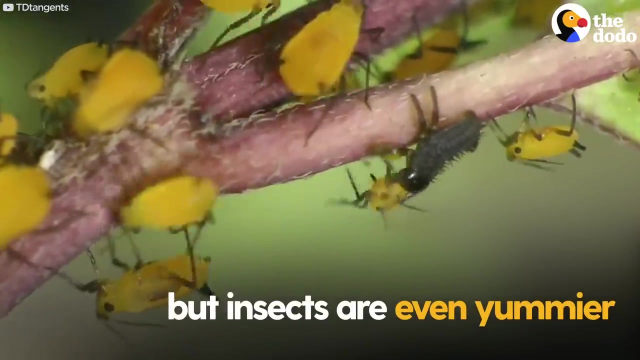 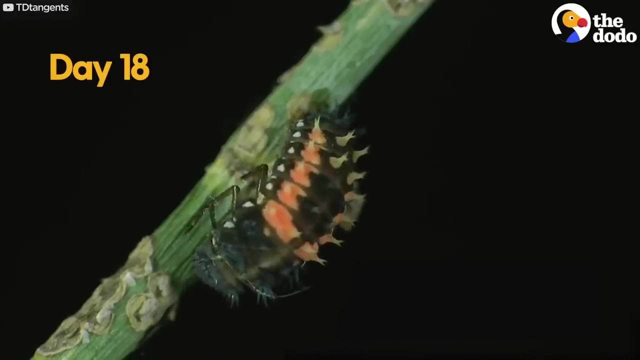 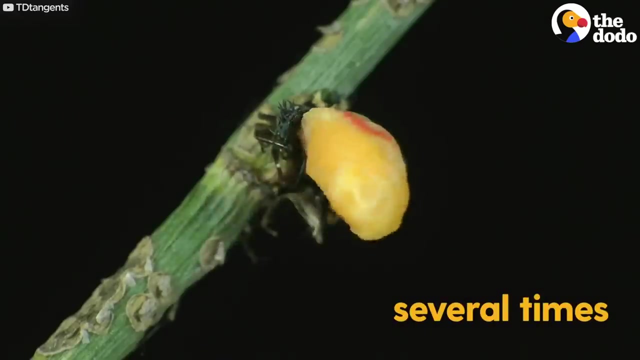 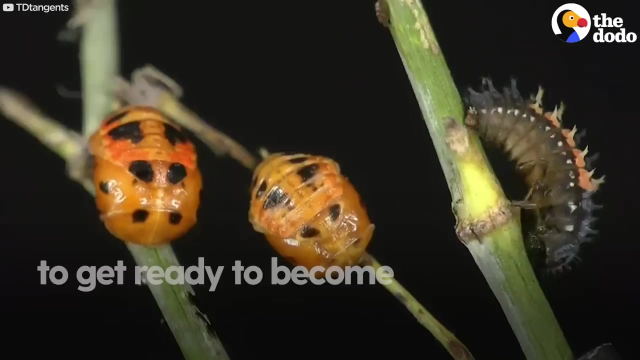 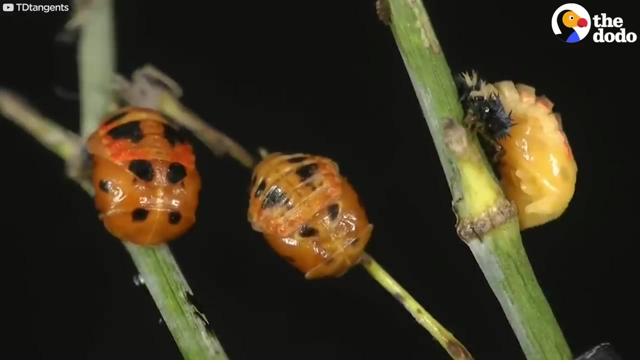 Please subscribe to the channel and press the bell icon to receive notifications when I upload a new video. Thank you very much for watching. Please like and subscribe. I'm glad you like it. See you next time. Bye-bye, Thank you. 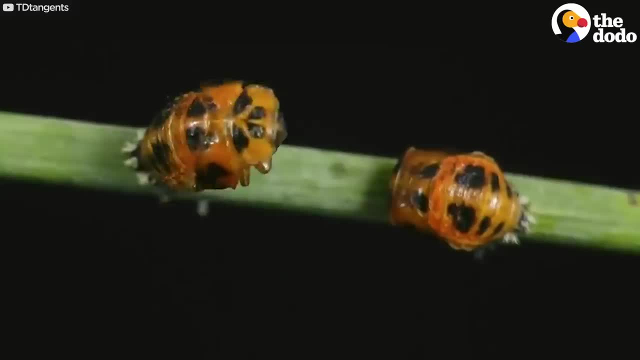 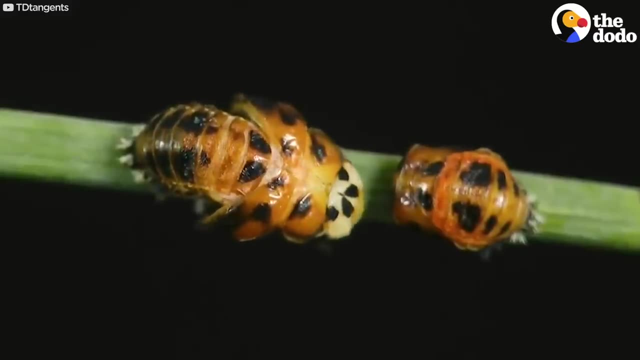 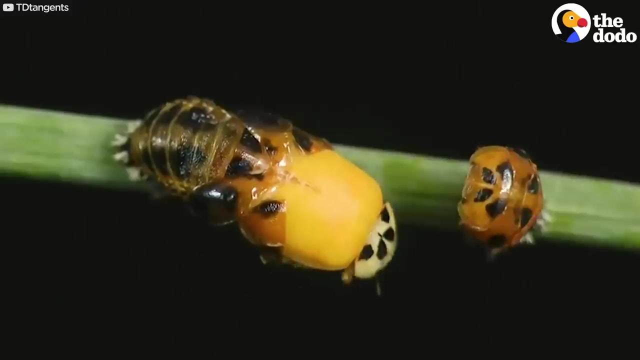 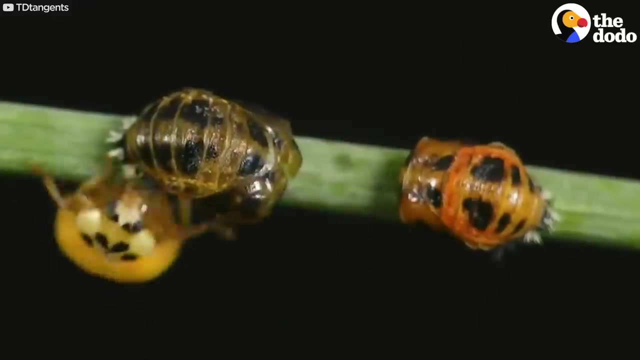 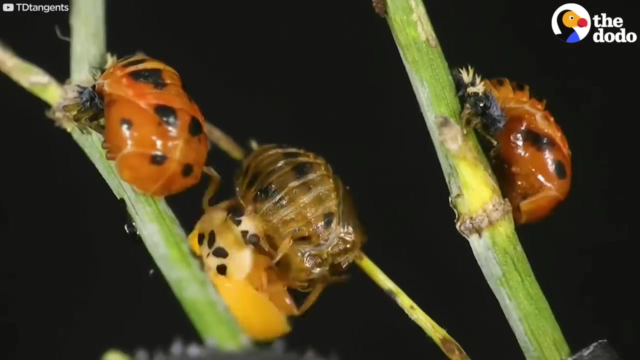 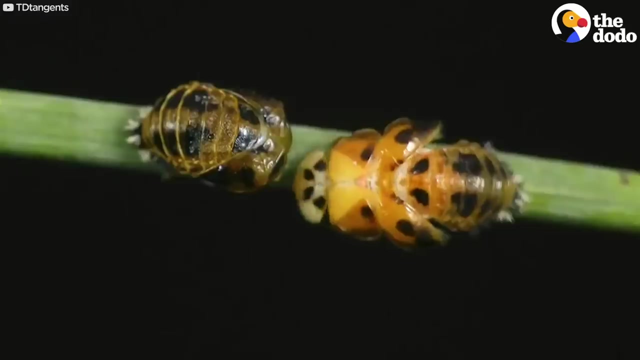 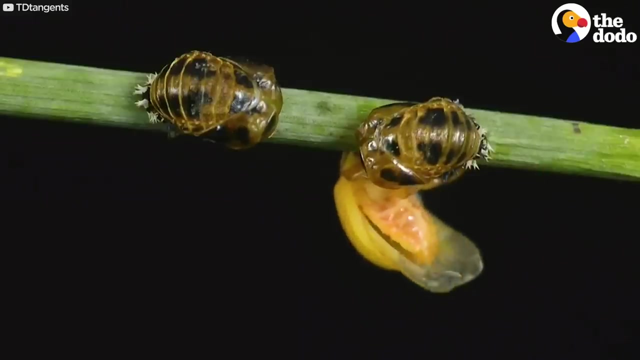 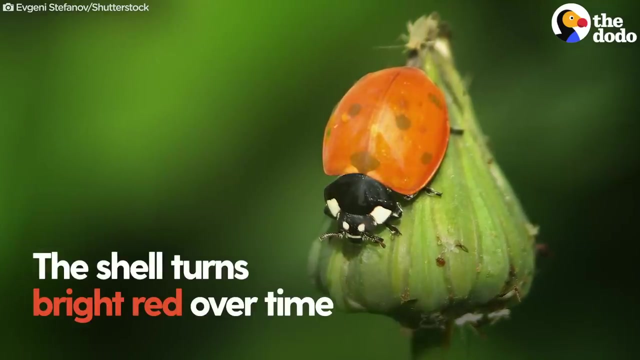 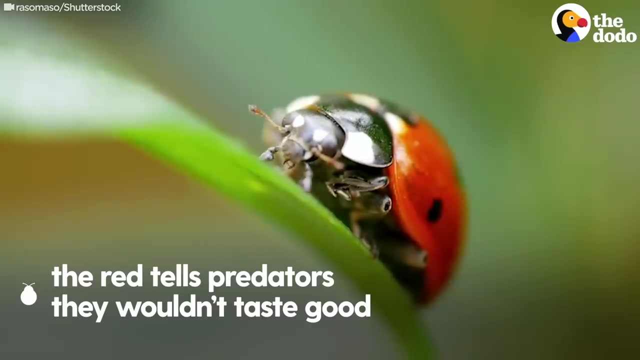 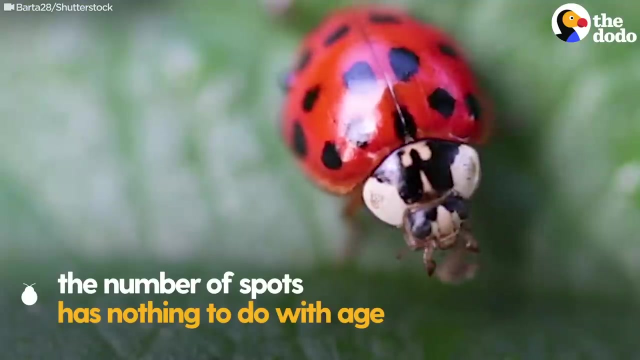 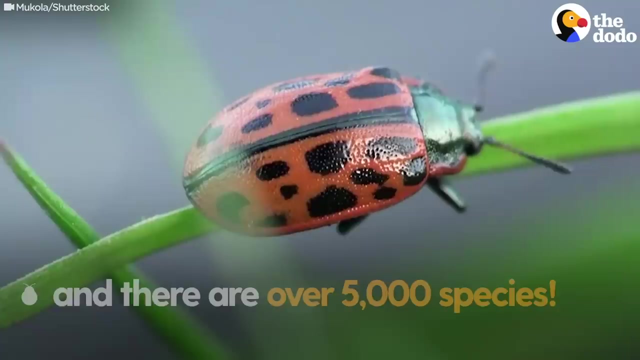 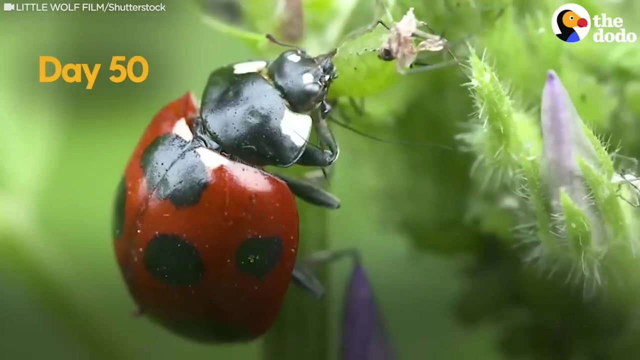 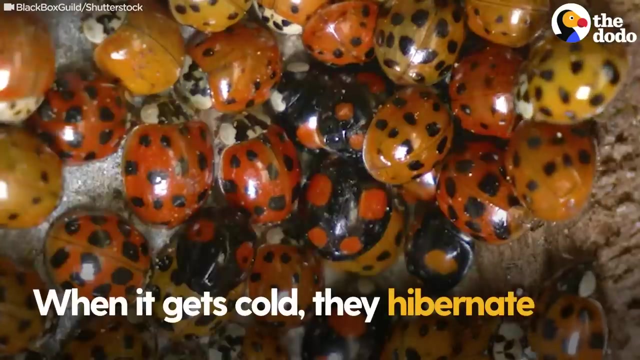 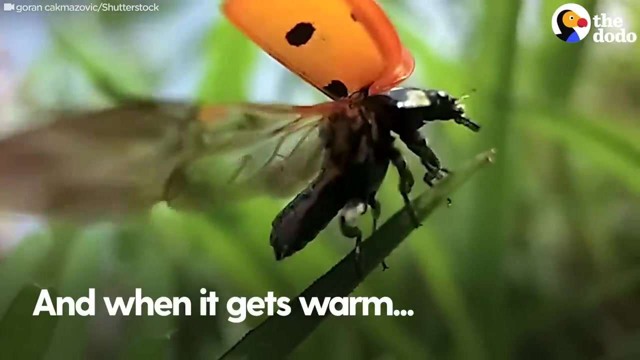 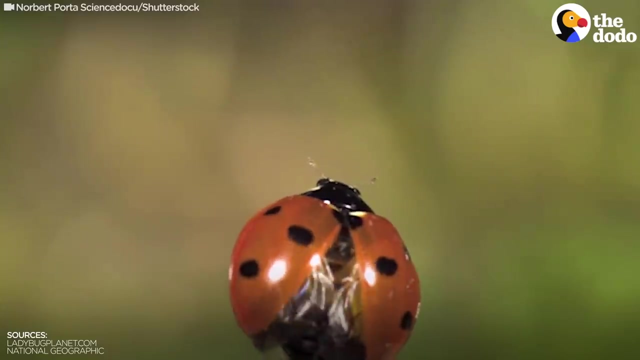 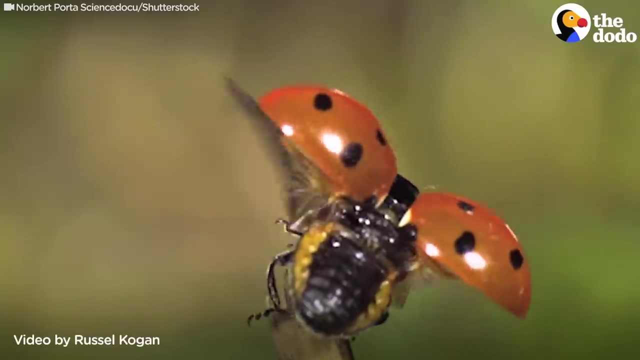 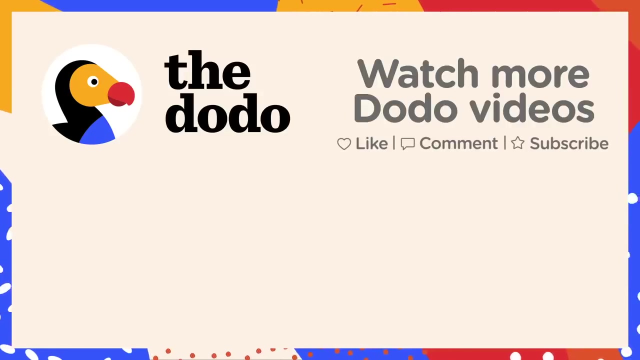